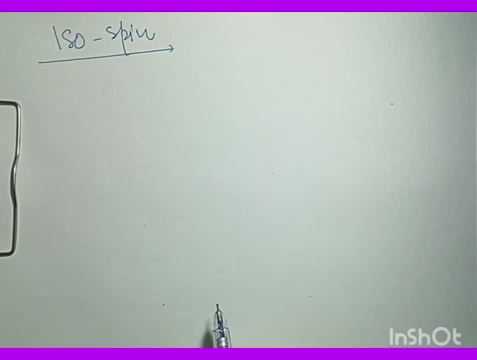 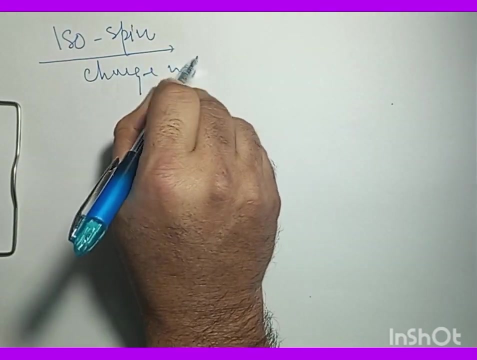 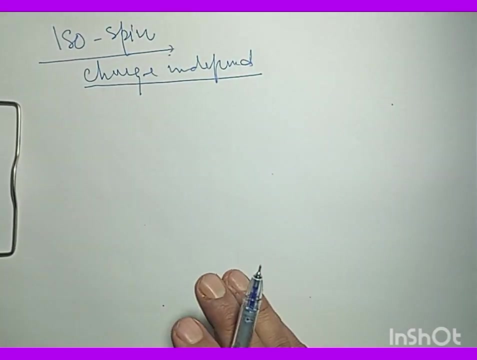 Now let's talk about isospin and probably its third component. Now what we have, what we talk about the nuclear force, is that this nuclear forces are, they are, charge independent. That means the force between proton-proton is same as that of the force between proton-neutron and neutron-neutron. 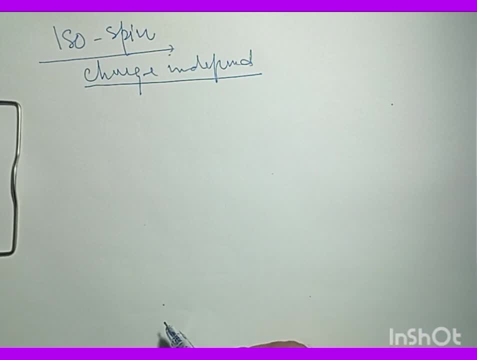 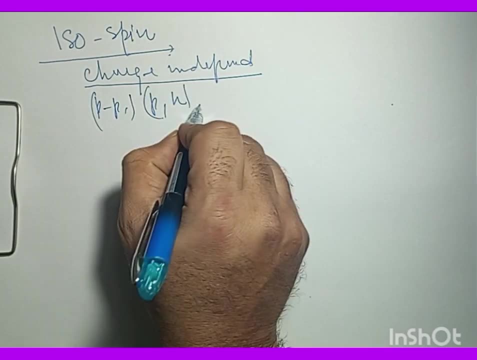 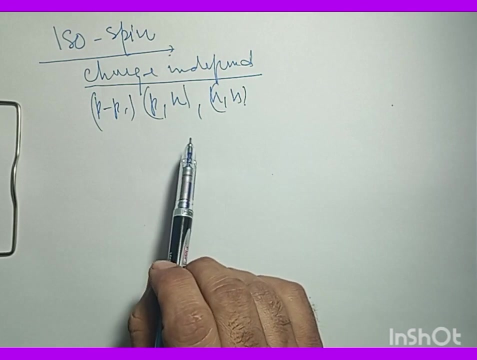 And so to say that these nuclear forces, between proton-proton and proton-neutron pair and neutron-neutron pair, all of these forces have the same force. They are the same magnitude And the charge independence of the nuclear force. it basically leads to the introduction of new quantum number. 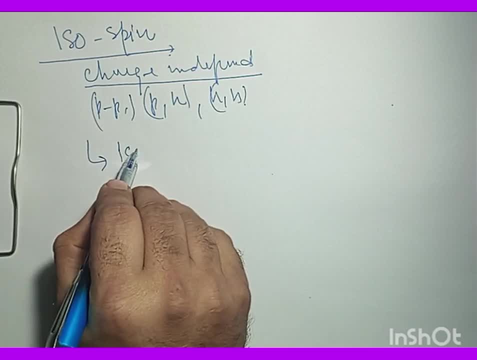 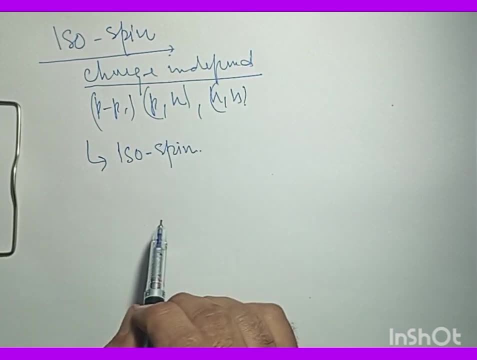 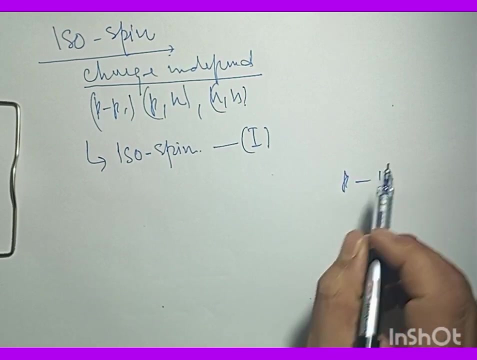 And this quantum number is called as what is the title of this subject here is isospin. So this isospin is a result of the independence of the charge of the nuclear forces And it was symbolized as I and it was- it was Heisenberg who considered that, that that proton and a neutron in a nucleus. basically they are the two states of a single particle. 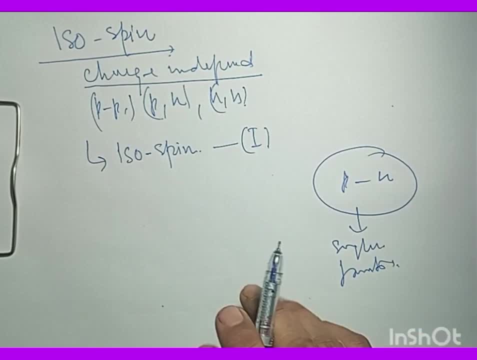 There are two states of a single particle, and, and that particle is called as nucleon. Now does these, these protons, the proton and the neutron in the nucleus are basically the, the two states of of this nucleon. 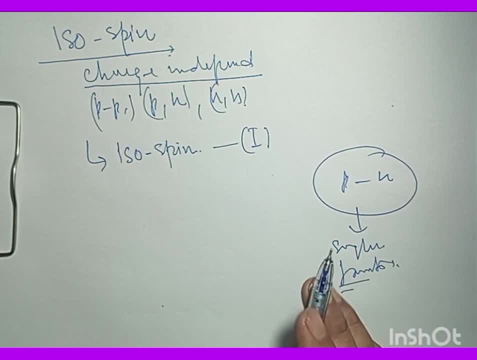 The, the two states of nucleon. they are described by isospin. They are described by by. by the space of isospin I mean internal charge space, or or or. we may call it isotopic spin, or or or by isobaric spin. 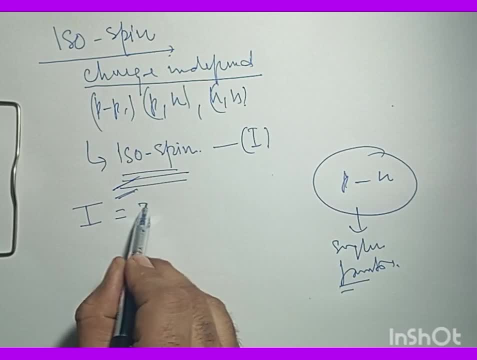 Now I is two I plus one orientations. These are the possible orientations. Now, now the nucleon of of this isospin I, if I take this, I is. it has one by two, How how much it has. it has basically two I plus one orientations. 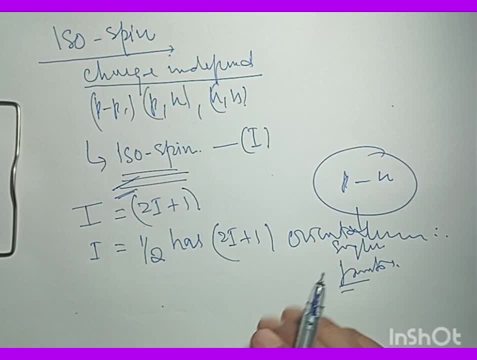 These are the possible orientations in isospin space, Now the three components of this isospin that we have. so if I take this, I equal to one. this is two times one by two plus one, so this is going to give me three orientations. 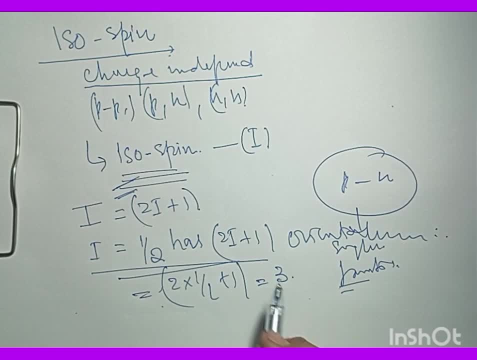 So we have, we have three components of this isospin, and these three components can be symbolized as I1, I2, and and I3.. And the value of I3.. The third component, that that I'm talking about here: what it does, it distinguishes. 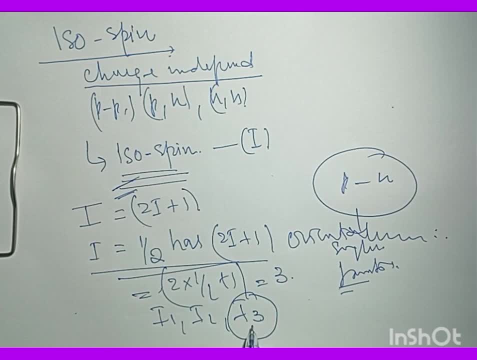 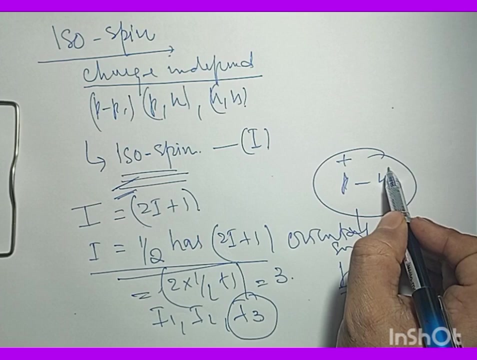 between proton and neutron And and the two states, that's proton and neutron of a nucleus. they have nearly same mass, but proton is positively charged, it has a positive charge, and and neutron does not have any charge, it's a neutral particle. 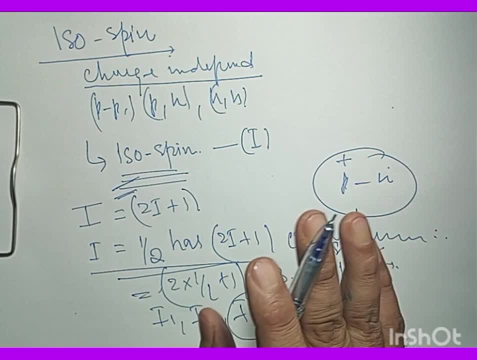 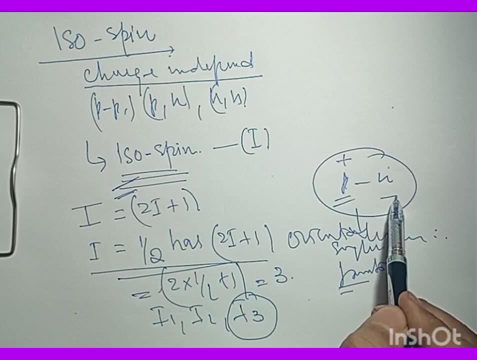 So hence, due to due to electromagnetic interaction, there is a slight mass difference between this proton and neutron. In other words, I would say that the mass of the proton is slightly different than that of mass of the neutron, And that's because of this electromagnetic interaction between these two. 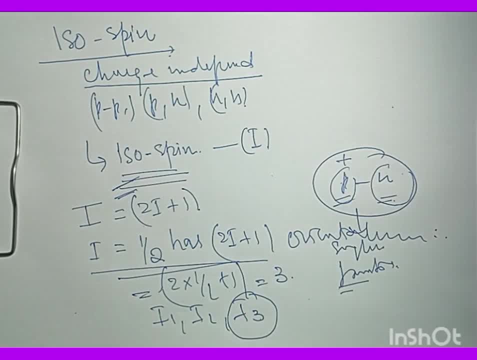 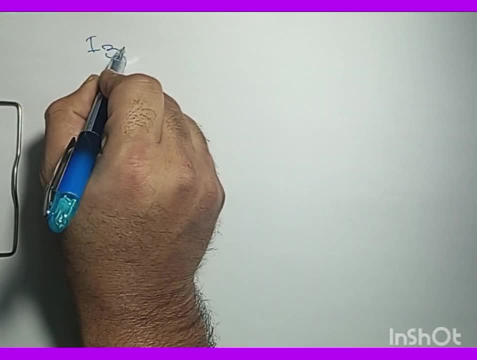 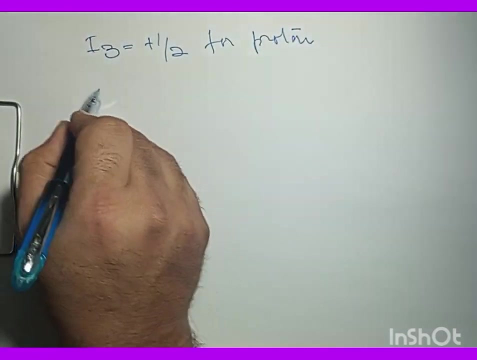 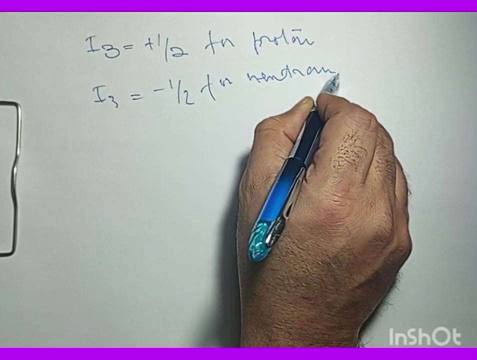 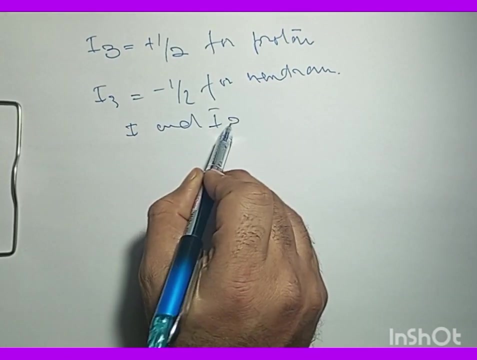 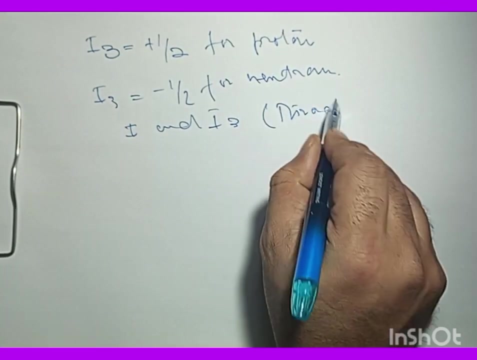 particles And now taking I3 equal to plus half for proton and taking this I3 as minus half for neutron, The value of I that we have and I3, for a given state of a particle. it can be written in Dirac notation. We can write down: 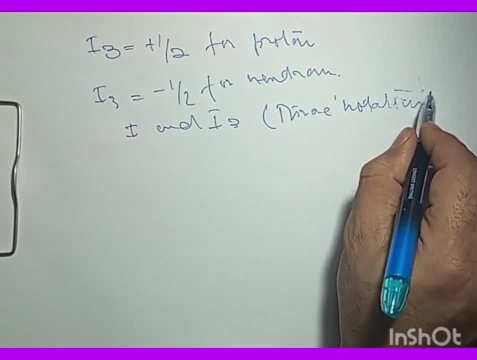 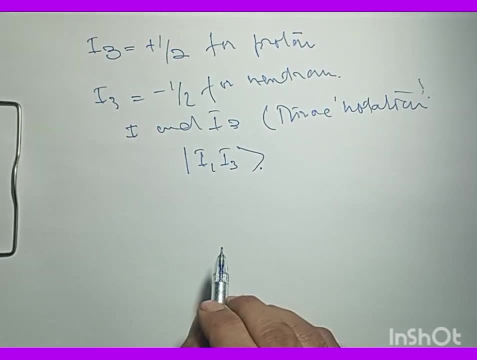 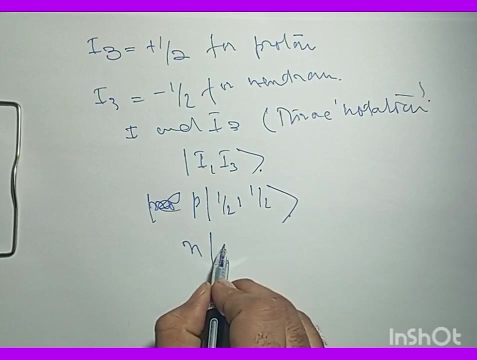 that in Dirac notation. So how we can write, We can write: I, I3, ket. So the proton and the neutron, I mean the two states of a nucleon, can be written. as for proton, so it is p. p. for proton it is 1 by 2 and it's 1 by 2, ket. For neutron, we have 1 by 2 and minus 1 by 2.. 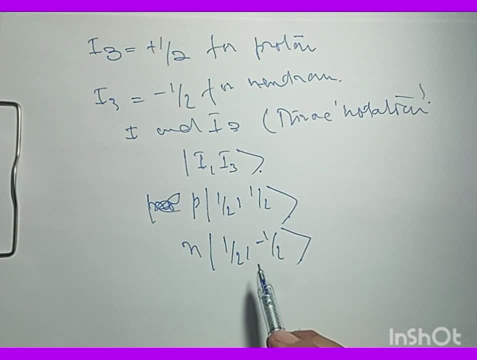 Okay, we have minus 1 by 2 for this And similarly, if we take pi massons, pi massons with isospin, I equal to 1.. So this implies we have 2s- sorry, 2i plus 1 possible orientations. This is 2 times 1 plus 1. 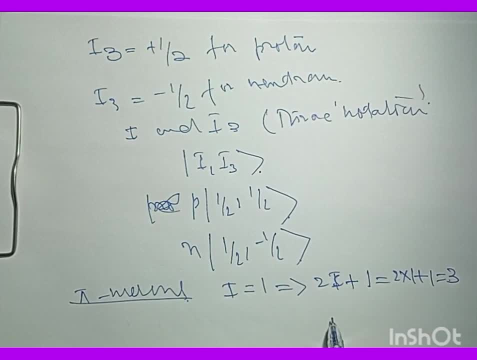 is equal to 3.. So there are three possible orientations in the isospin space. Now the values of I3 for the different orientations for this, this masson. So we can have I3, it's plus 1 for Pi positive massons, It is minus 1 for Pi negative masson And it is 0. 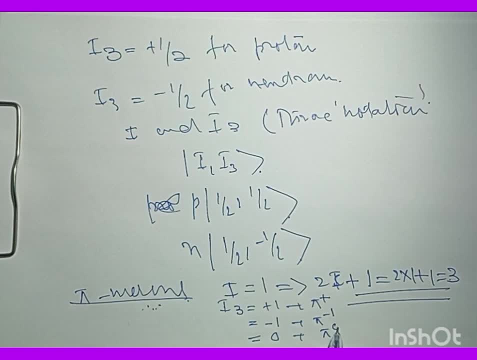 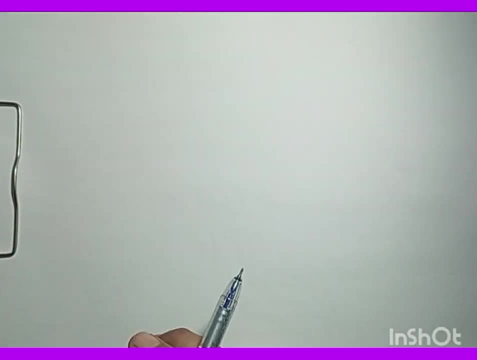 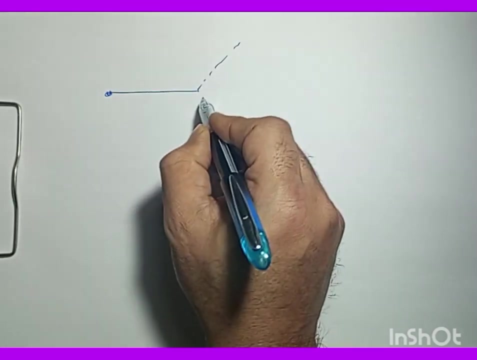 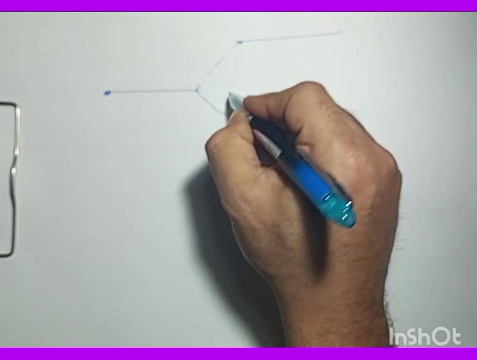 for Pi zero massons. Now let's try to figure out, let's draw these states of. what we have is we have a nucleon state and this nucleon state is breaks down into two states, and the two states are a result of electromagnetic. 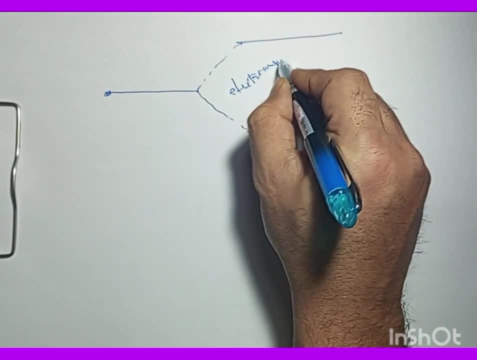 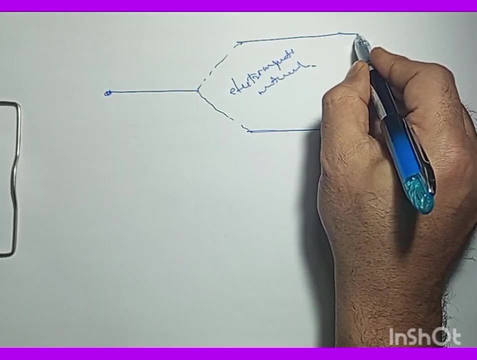 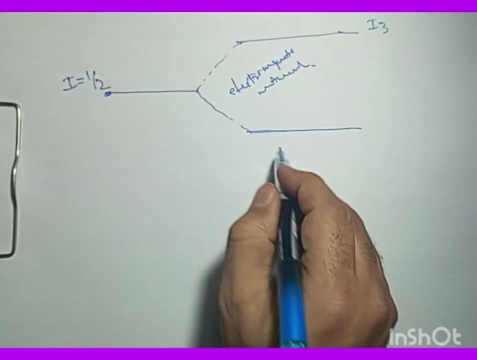 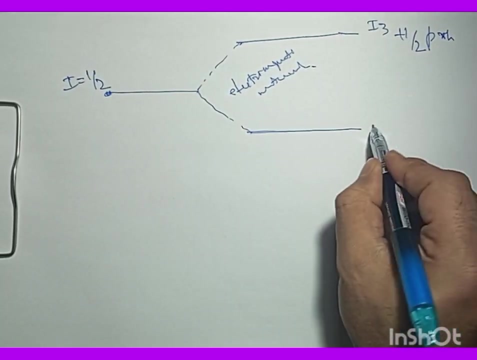 interaction, electromagnetic interaction and what we have here. here we will have I3 states. so here I have: I equal to 1 by 2, so what I'll have is plus 1 by 2 state, that's for the proton, basically, and minus 1 by 2 state for the neutron. now 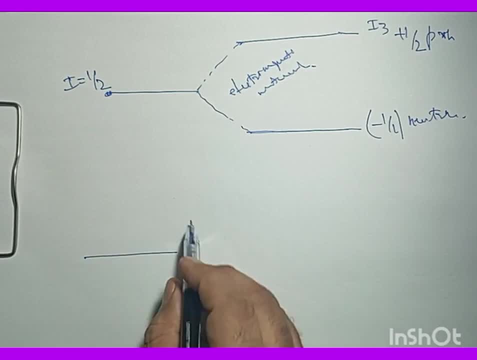 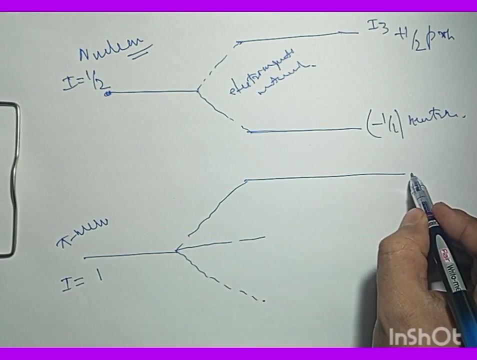 similarly talking about a pi masson. so for pi masson we have three states: 1, 2 and and 3. so I for masson is 1, so this is for pi masson and and this is for nucleon. ok, so what we will have here is minus 1 by 2, that's for neutron. this is no minus. 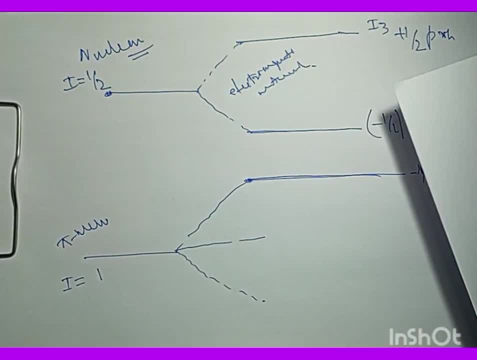 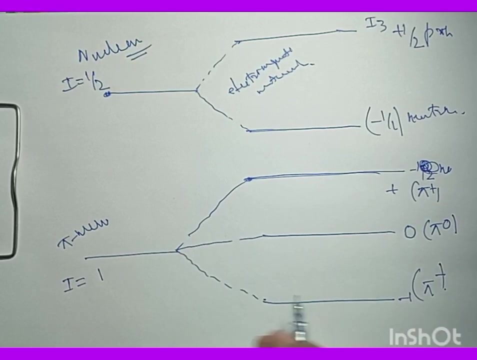 1 by 2. there we have plus 1, minus 1 and 0. so for plus 1 we will have pi plus masson and for 0 we will have pi neutral masson and for minus 1 we will have pi minus masson. and to write down the total charge and 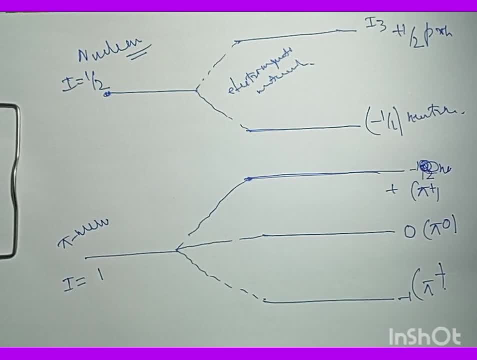 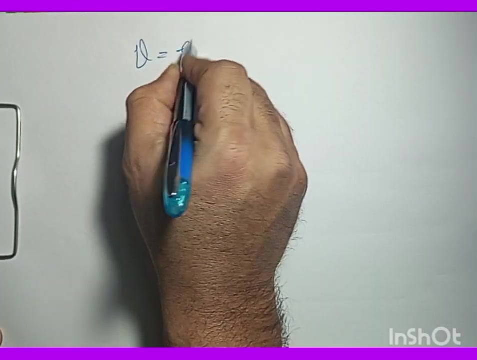 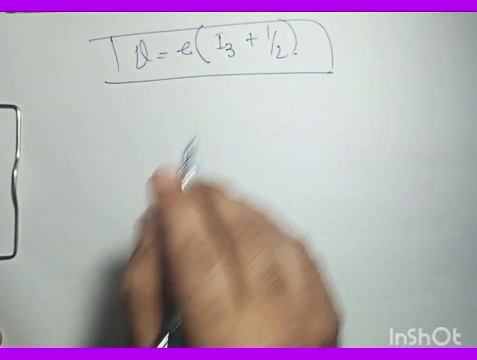 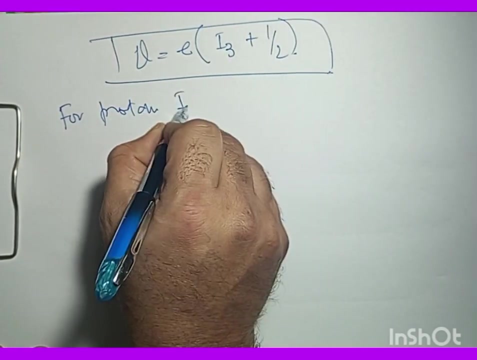 the electric charge on the state of the particle, having this get state, what cat state we have I I3, cat. for this state to write down, the charge, Q is e times i, 3 plus 1, 1 by 2.. So for a proton, if I take for proton, what is I3? I3 is plus half and therefore what will be the charge? 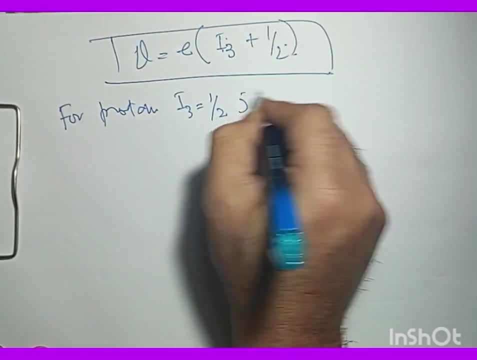 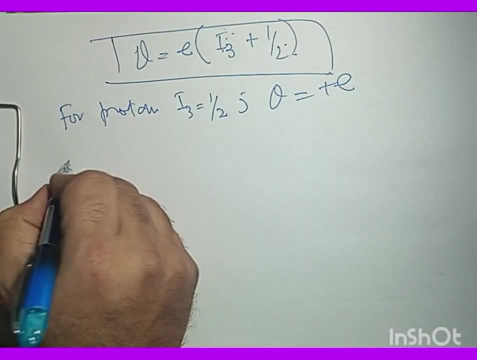 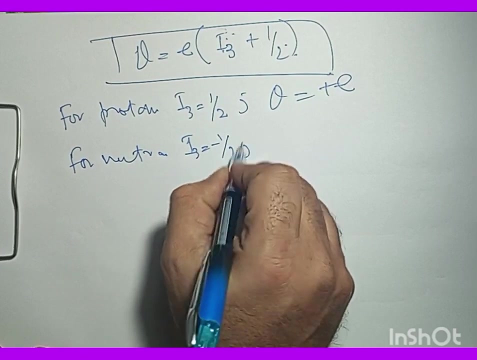 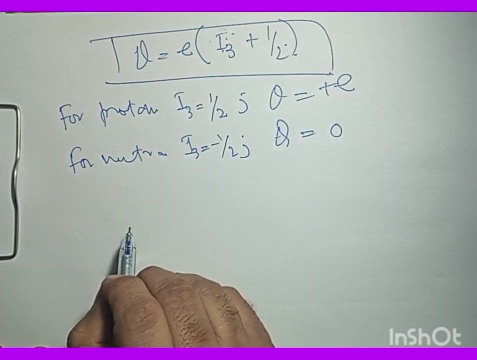 So if it is half half plus half will give us Q equal to plus E, simply because putting I3 equal to 1 by 2 will give us 1.. Now for neutron, what we have we have I3 is minus 1 by 2, and minus 1 by 2 and plus 1 by 2 will cancel, for neutron will have a charge Q equal to 0. 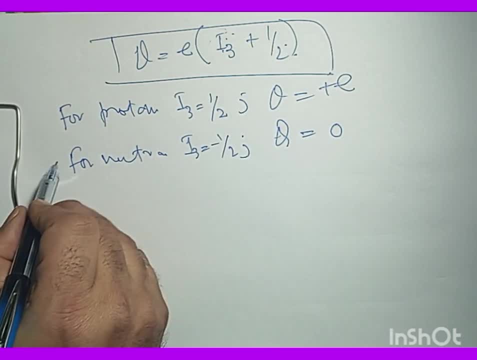 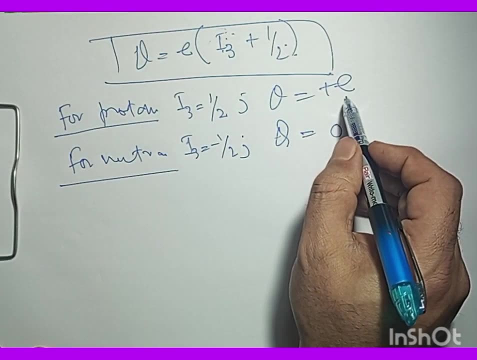 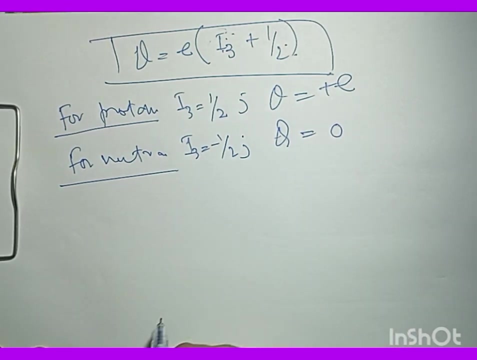 So the isospin, the isospin for the proton and neutron, and talking about the charge of the proton, is positive And the charge of the neutron is negative. Now let me tabulate this thing. Let me tabulate this isospin and its corresponding third component, I3, that we talked about here, for nucleons, mesons and also for hyperons. 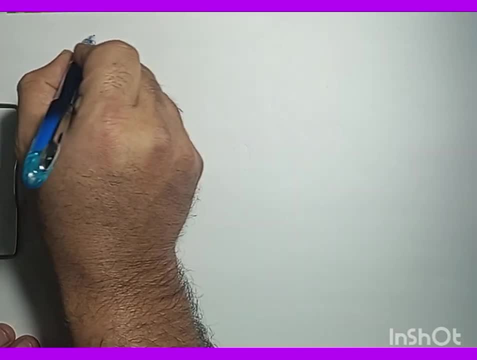 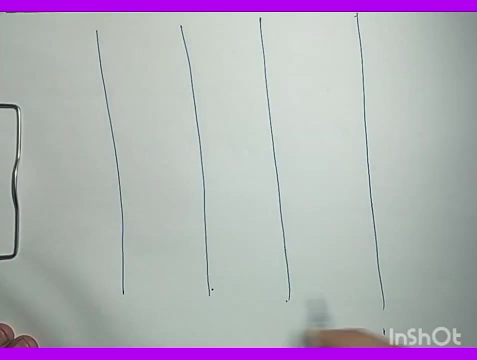 So let's go with that. So what we will have, we will have the family, then we will have the particle, then we will have its antiparticle, then we will have the isospin And then we will have the third component. 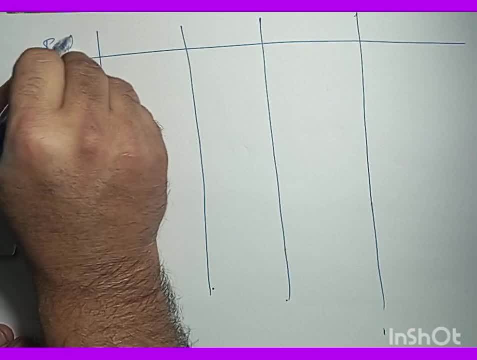 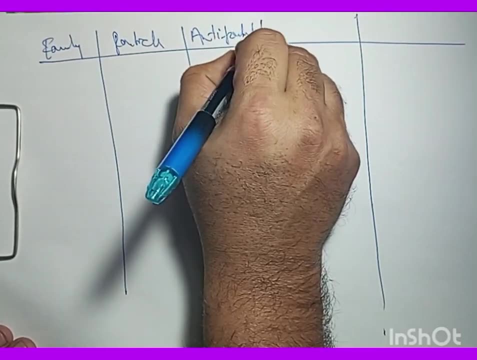 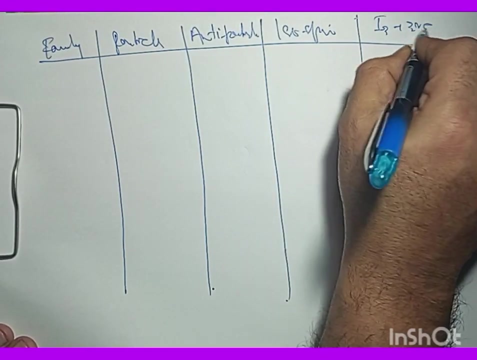 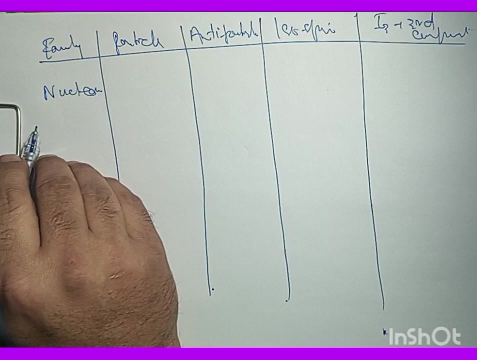 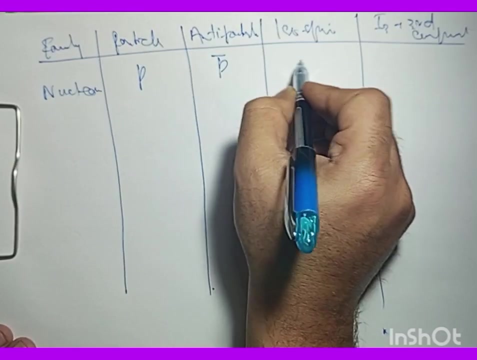 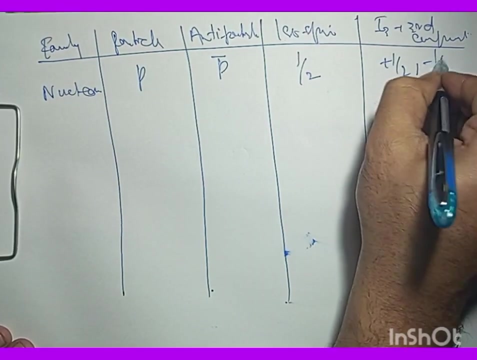 So what we will have? we will have family and particle, antiparticle, isospin and I3, third component. third component: Now let us start with the nucleons. So nucleons, okay, we have protons And its antiparticle is P bar and its isospin is half and its third component is plus half and minus half. 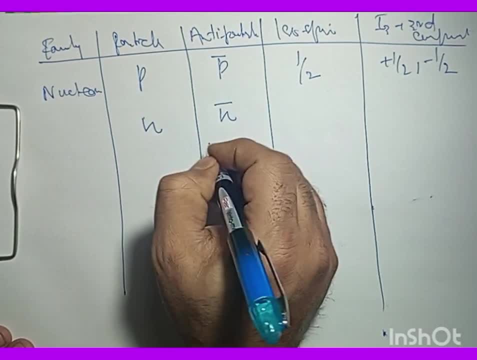 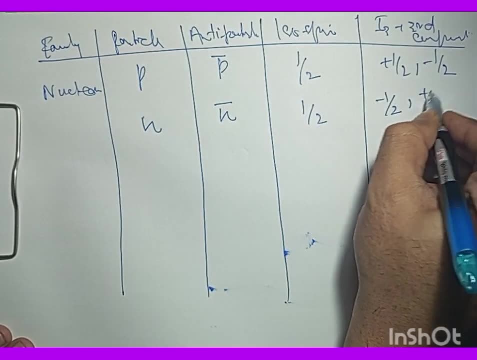 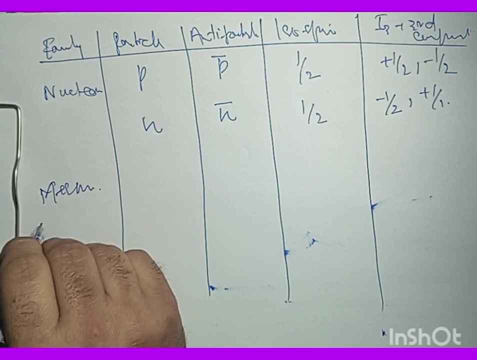 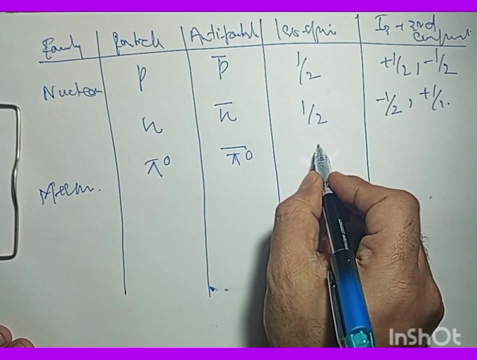 Now talking about neutron, we have antineutron. its antiparticle, isospin is half and it is minus. third component is minus half and plus half. And now talking about mesons, So we have pi neutral. we have pi neutral, bar its antiparticle, and it has an isospin of one. 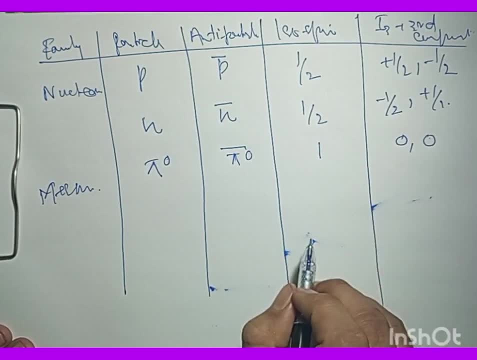 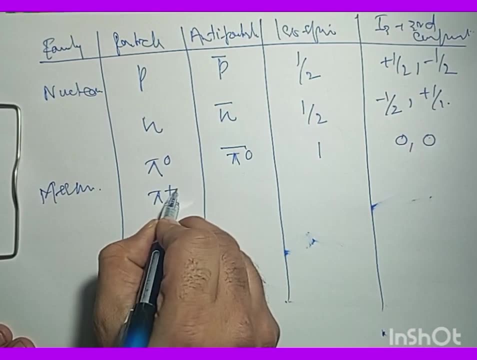 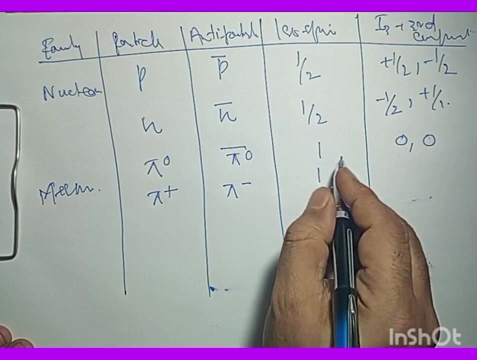 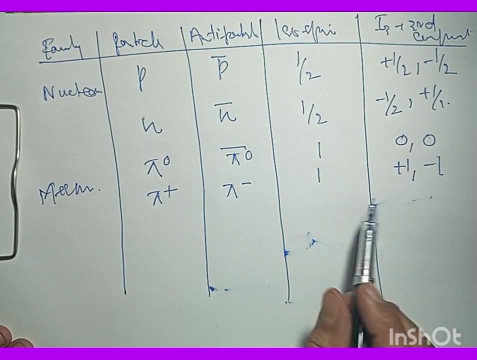 So its I3 state is zero And pi positive, its antiparticle is pi negative and its isospin is one And it has plus one as minus one the I3 states. So plus one is for the pi plus and minus one is for its antiparticle. 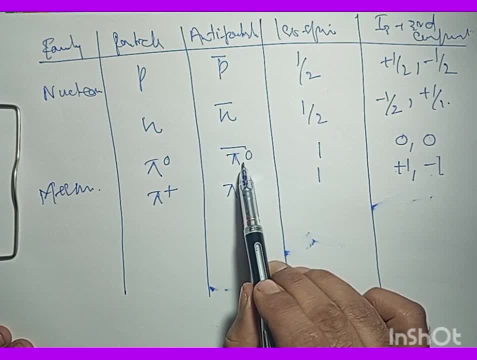 And zero is for pi zero and zero is for its antiparticle, Minus one by two is for neutron I3 component and plus one by two is for the antineutron. And going with K plus For K plus, we have antineutron. 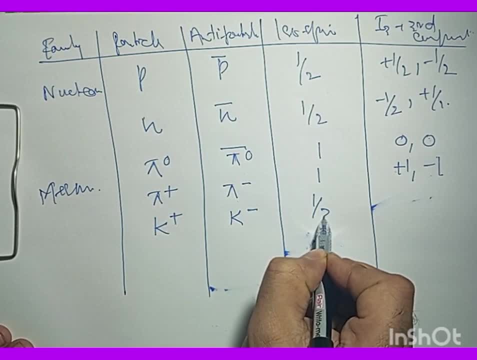 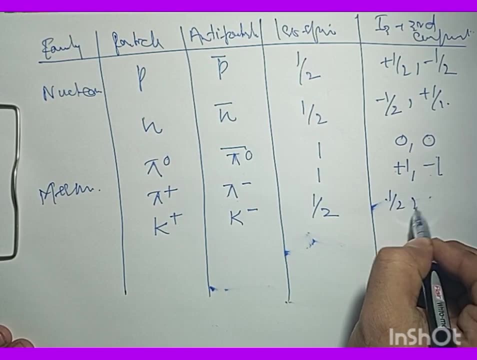 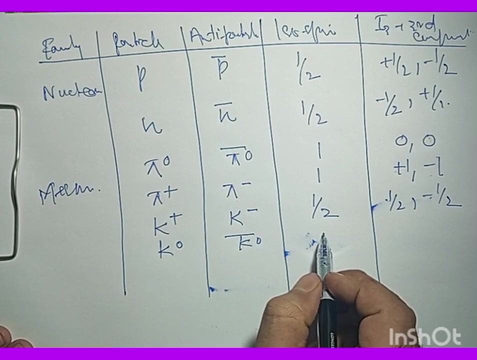 So this is anti-K minus. it has an isospin half. So we have I3 component for this. K plus is one by two comma minus one by two. And similarly, if we take K zero, it's K zero bar, K neutral bar and it has an isospin of half. 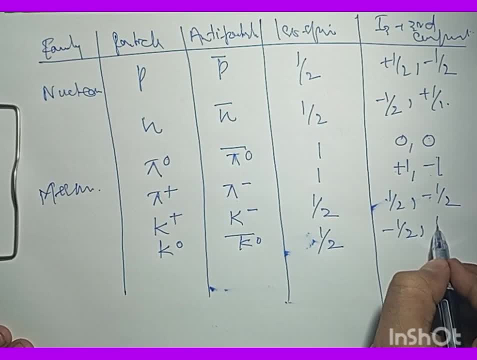 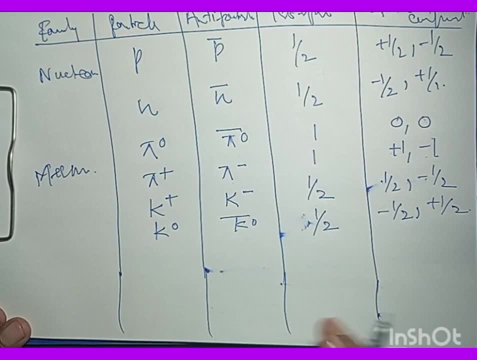 So this is minus one by two and plus one by two. Now, going with sigma particles, Sigma sigma positive- we have sigma positive bar and its isospin is one and the I3 components for sigma plus and its antiparticle is plus one and minus one. 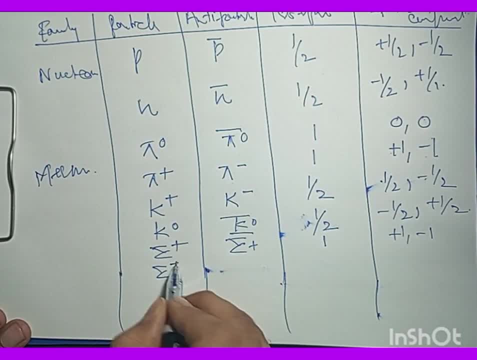 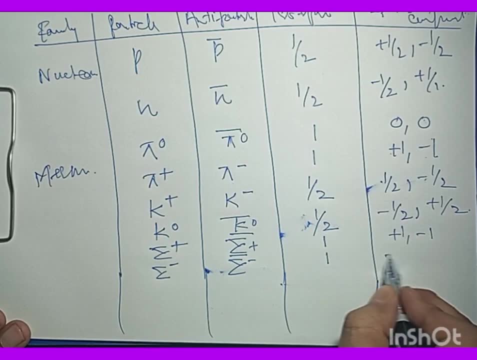 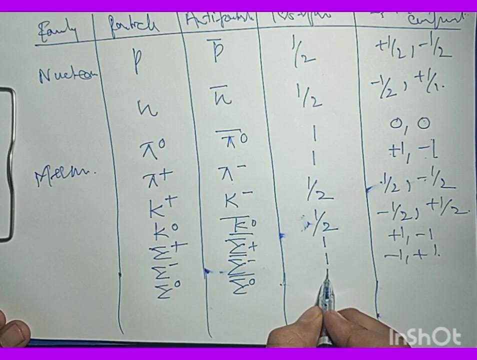 And similarly for sigma minus. we have sigma minus bar, and we have one here, And and we have minus one and plus one as their I3 components. And sigma zero is sigma zero, bar is its antiparticle and it has isospin of one and its I3 components for both of them is zero and zero. 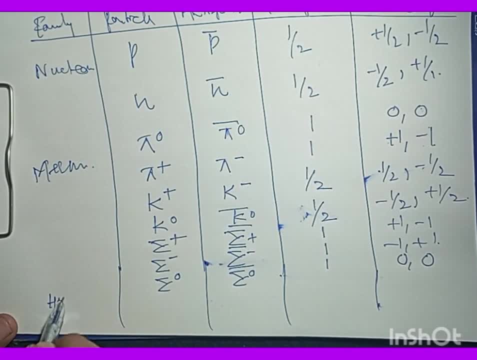 And after this we have hyperons. We'd like to write down hyperons For hyperons. We have lambda, neutral lambda bar and it has a spin of zero and zero, zero. And then we have chi minus. So this is chi minus bar and isospin is half. 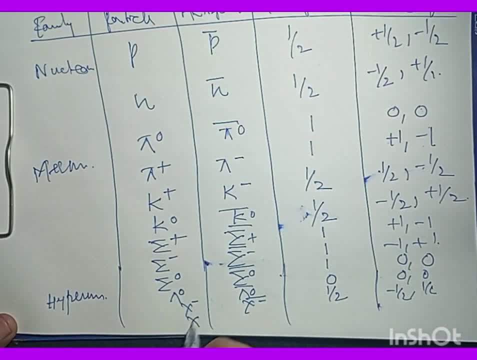 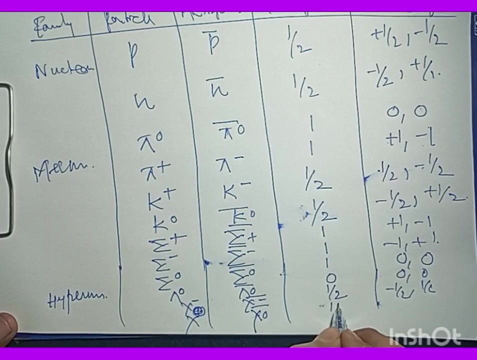 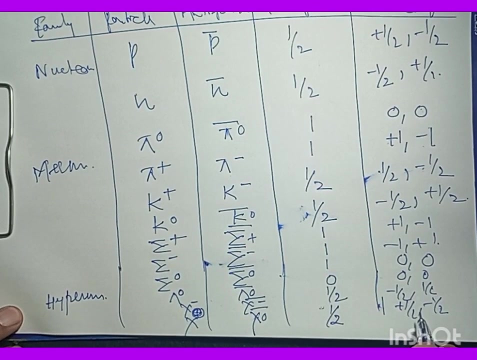 So this is minus half and half And chi positive. Then we have no, we have chi neutral here. So chi neutral then chi neutral bar. that's going to give us one half is its isospin and plus half and minus half are the I3 components for chi neutral and its antiparticle chi neutral bar. 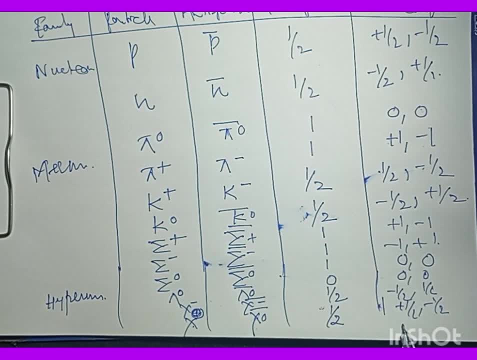 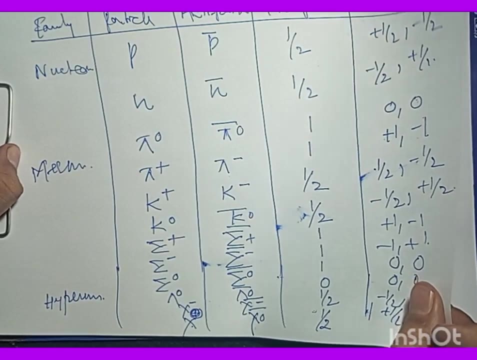 And its isospin is half And and the I3 components Are plus half and minus half. Now we have a relation here between electric charge and third component of this isospin and isospin I3 and the baryon number. 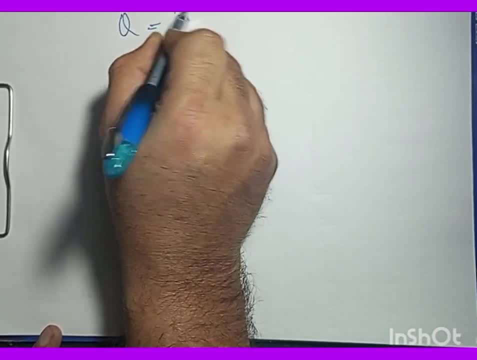 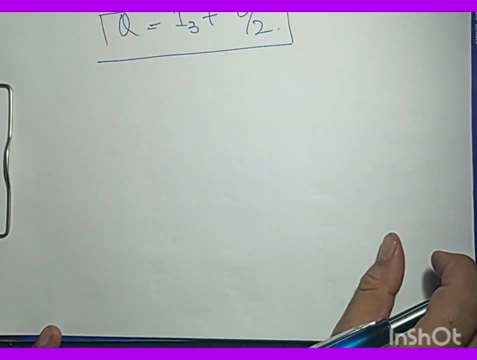 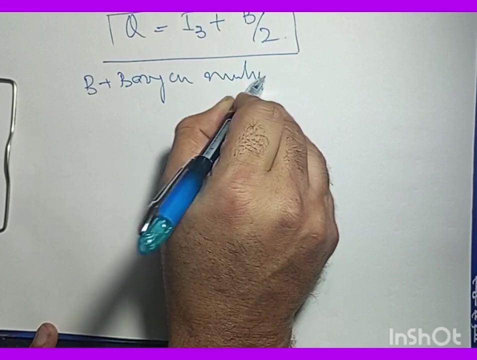 So what's that relation? is that charge is I3.. It's the third component plus the baryon number by two. All right, Well, B is the baryon number, And and Q is the charge and I3 is the third component. 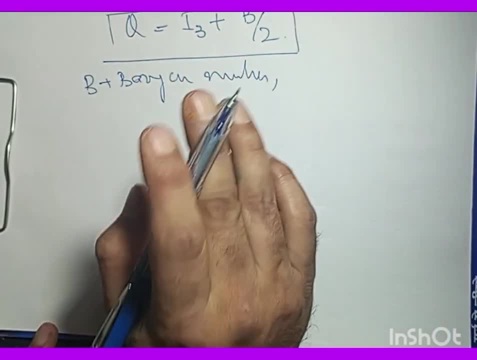 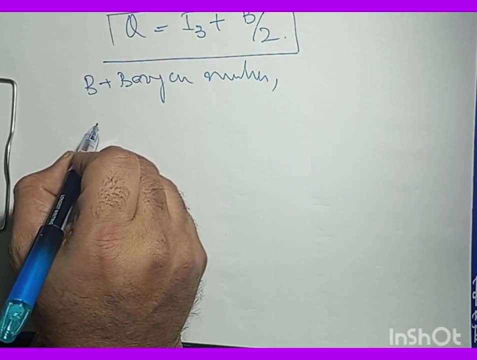 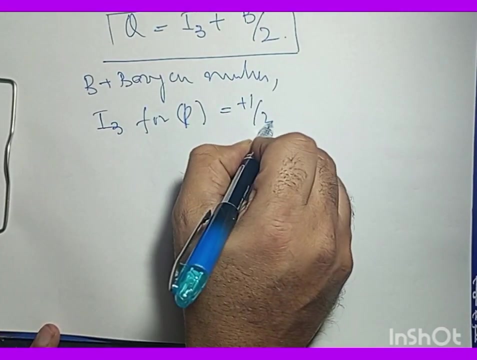 Now this relation is used to find the charge on each number of isospin multiplet. Now, for example, if I say that I3, I3 for for proton, if I, if I take it plus half, and B is plus half, 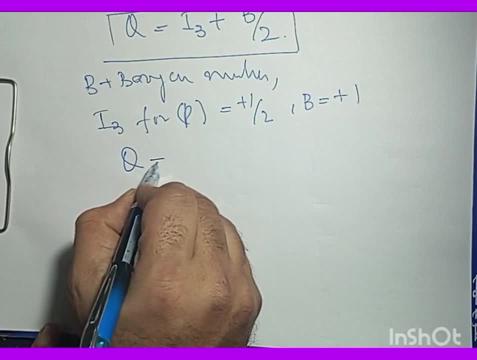 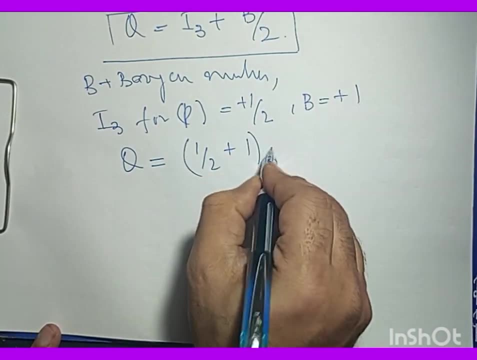 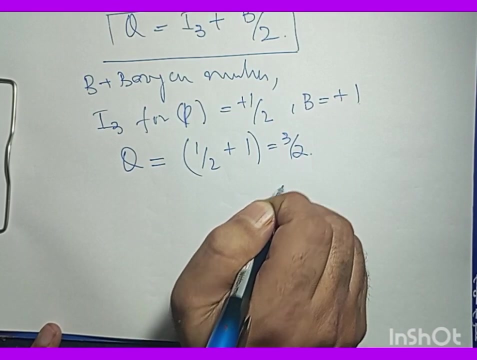 So what will be the charge in that case? So charge is going to be I3 is is one by two plus one, So that's going to be three by two. So the charge that we will obtain here, the charge on the proton. I think I have committed mistake here. 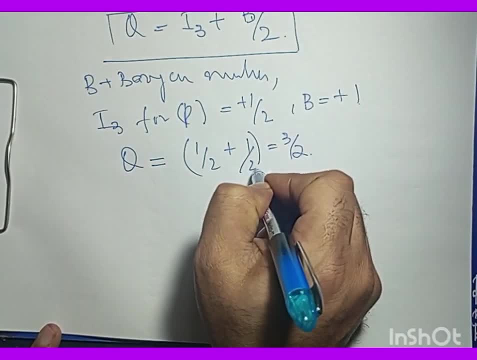 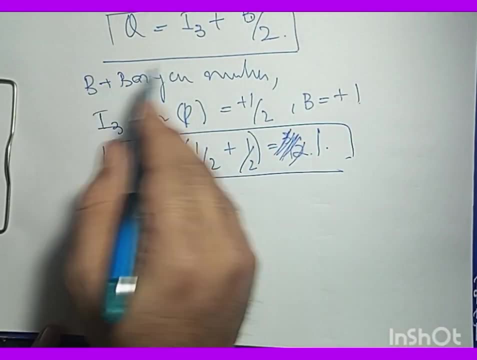 So this is B by two, So it is going to be one by two. So charge of proton is not fractional, So it is one. So using this equation of charge with baryon number and third component of isospin, we 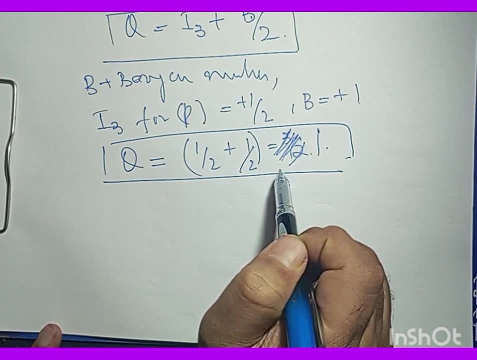 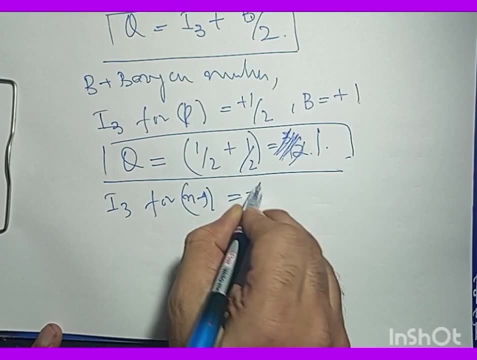 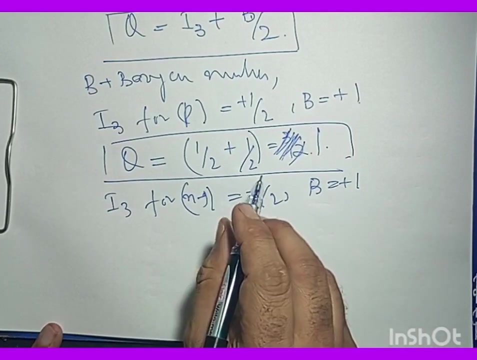 can calculate the charge of the proton, and this charge is simply 1.. And if we say for I3, now I3 for neutron, what's that? I3 for neutron is minus half. It is minus half and its baryon number is plus 1.. 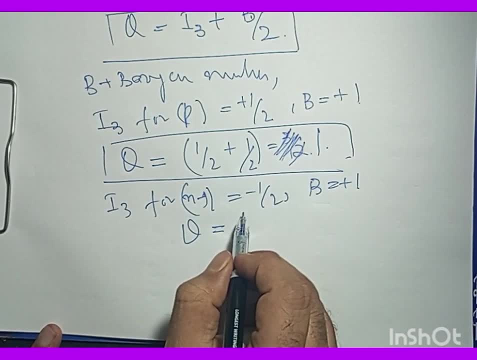 So what we are going to get here is Q. is so what we will have for I3, I have minus 1 by 2 and this is plus 1 by 2, the 2 will cancel and this Q will come out to be 0. 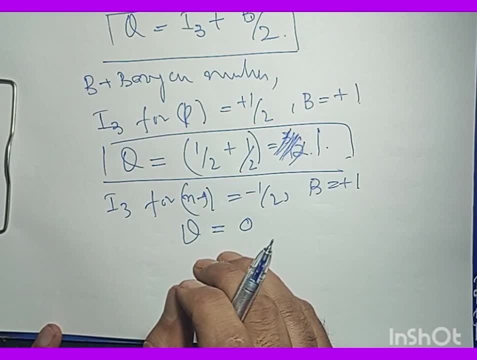 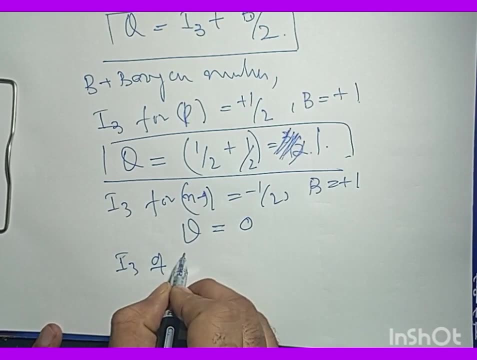 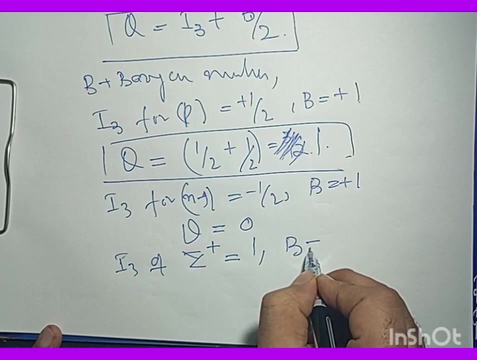 So we can say here that the net charge on the neutron is equal to 0. And similarly, suppose I take the I3 of sigma positive. The I3 of this sigma positive is 1. And the baryon number is plus 1.. 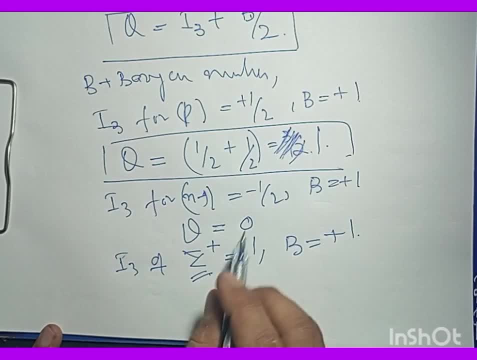 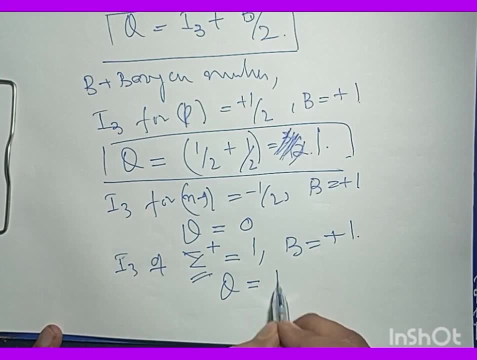 So what's going to be the charge of this sigma plus in view of this equation? So Q is going to be I3 is 1 for it. This is 1 plus 1 by 2. So that's going to be 3 by 2.. Okay, So that's it.